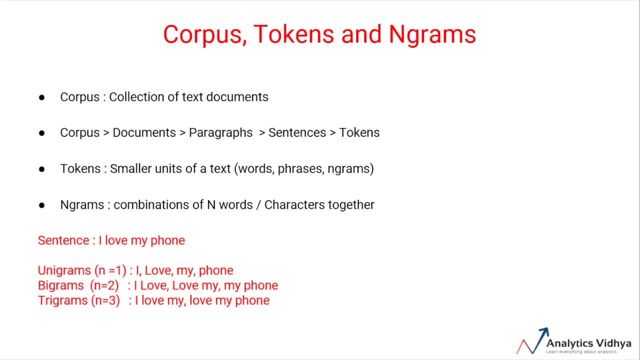 are I love love my my phone. And trigrams are I love my, love my phone. So unigrams are representing one words, bigrams are representing two words together and trigrams are representing three words together. Engrams are very useful in text classification tasks which we will. 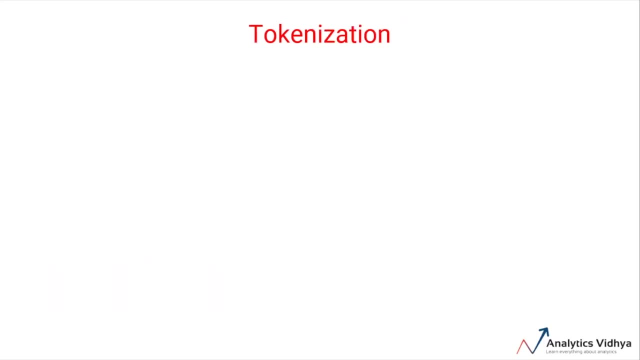 discuss in the later videos. Let's discuss about tokenization. Tokenization is a process of splitting a text object into smaller units, which are also called tokens. Example of tokens can be words, numbers, engrams or even symbols. Most commonly used tokenization process is the white space tokenization. In this process, 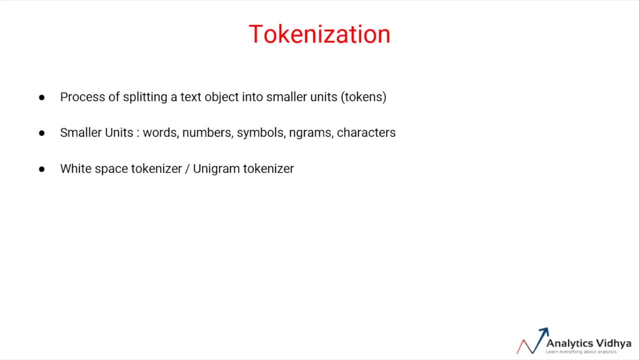 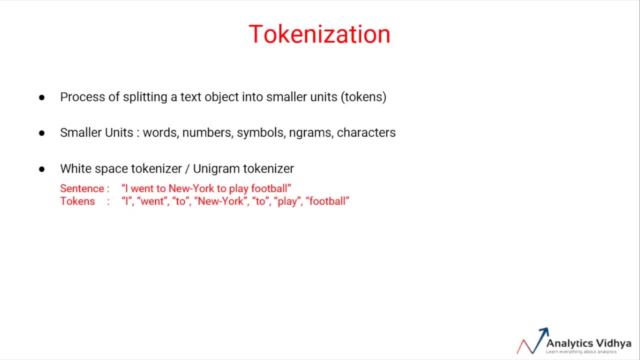 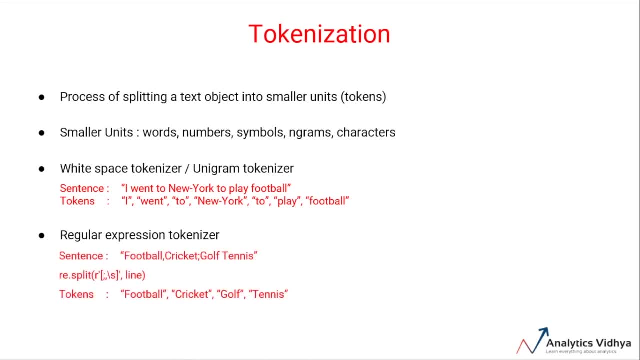 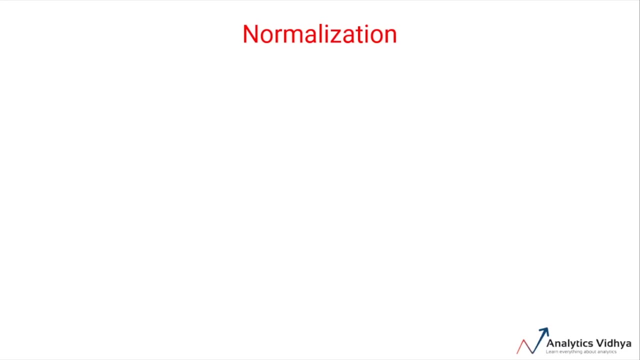 string containing multiple delimiters. We can split the text by passing a splitting pattern. Tokenization can be performed at the sentence level or at the word level, or even at the character level. is normalization? In the field of linguistics and NLP, a morpheme is defined as the base form. 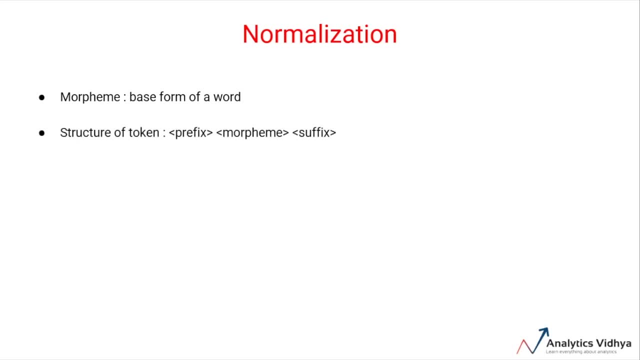 of a word A token is generally made up of two components: morphemes, which are the base form of a word, and inflectional forms, which are essentially the suffixes and prefixes added to morphemes. For example, consider a word antinationalist, which is made up of anti and. 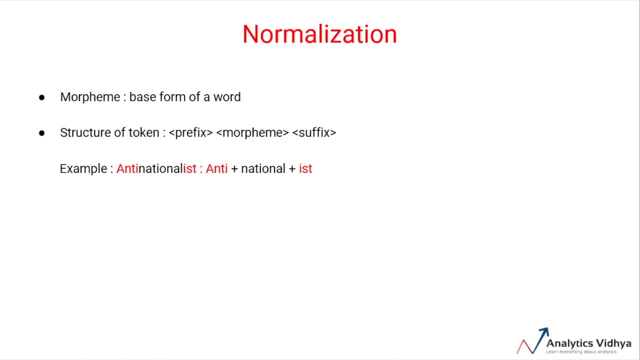 IST as the inflectional forms and national as the morpheme. Normalization is the process of converting a token into its base form. In the normalization process, the inflectional forms from a word are removed so that the base form can be obtained, So the normalized form of 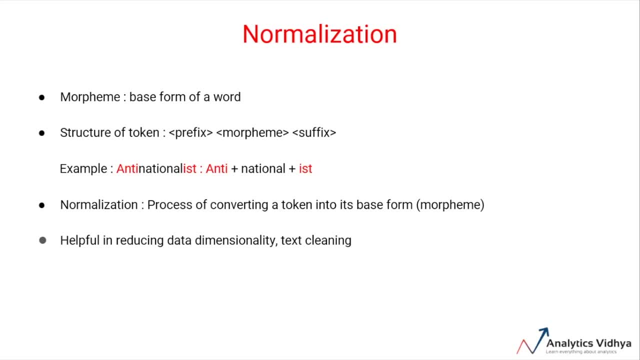 antinationalist is national. Normalization is useful in reducing the number of unique tokens present in a text, removing the variations of a word in a text and removing redundant documents information. Two popular methods which are used for normalization are stemming and lemmatization. 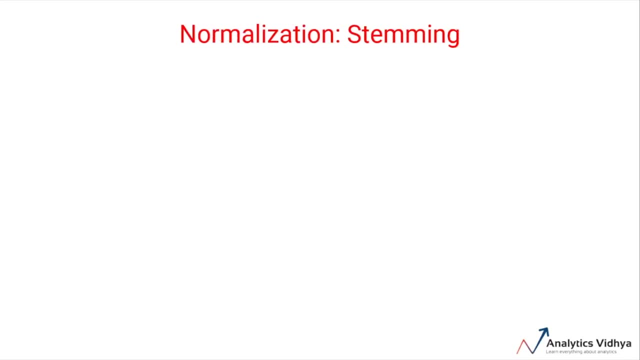 Let's discuss about them in detail. First of them is stemming. It is an elementary rule-based process for removing inflectional forms from a token and the outputs are stem of the word. For example, laughing, laughed, laughs, laugh will all become laugh because their inflectional form 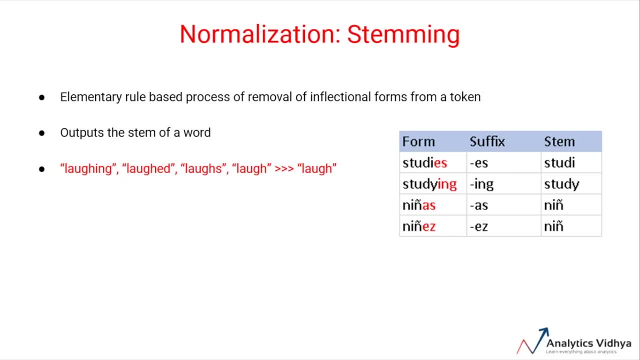 will be removed. Stemming is not a good normalization process because sometimes stemming can produce the words which are not present in the dictionary. For example, consider a sentence: His teams are not winning. After stemming, the tokens we will get are: hi- team are not win, and notice that the keyword win is not a regular word and hi changes the. 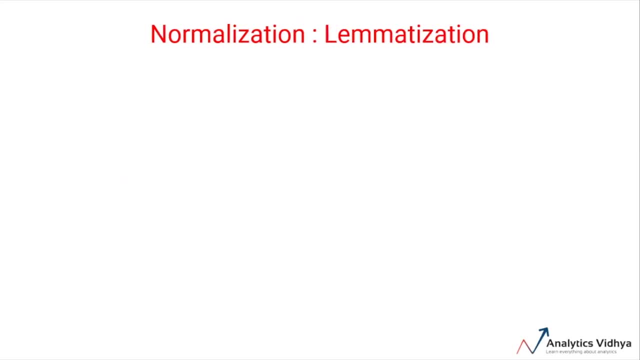 context of entire sentence. Lemmatization, on the other hand, is a systematic, step-by-step process for removing inflectional forms of a word. It makes use of vocabulary, word structure, part of speech, tags and grammar relations. The output of lemmatization is the root word called lemma. For example, am, are, is, will be. 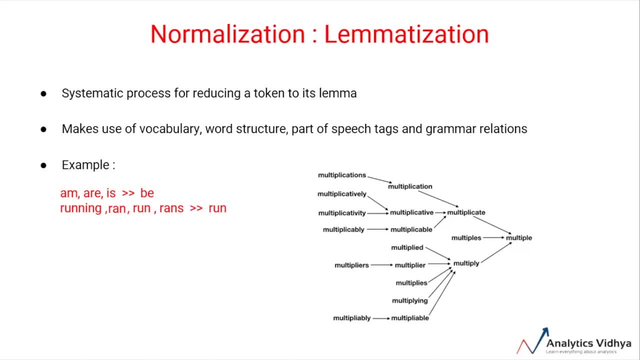 converted to be Running. ran, run rants will be converted to run. Also, since it is a systematic process, while performing lemmatization, one can specify the part of speech tag for the desired term, And lemmatization will only be performed if the given word has. 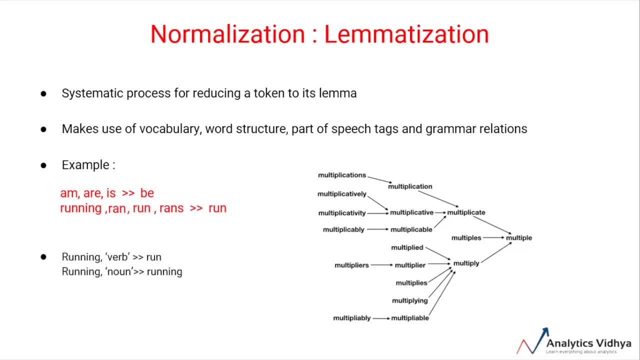 the proper part of speech tag. For example, if we try to lemmatize the word running as a verb, it will be converted to run, But if we try to lemmatize the same word running as a noun, it won't be converted. In the next video we will be talking about syntax and 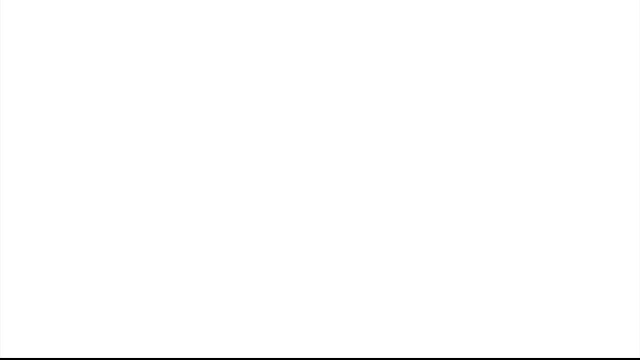 structural properties related to text. Thank you, Thank you.